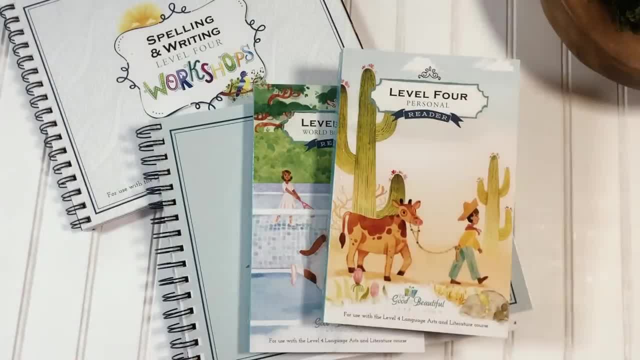 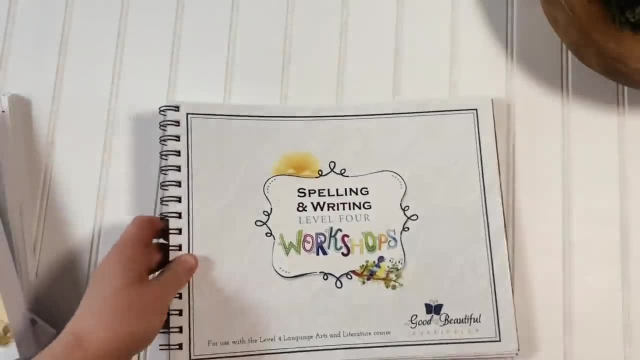 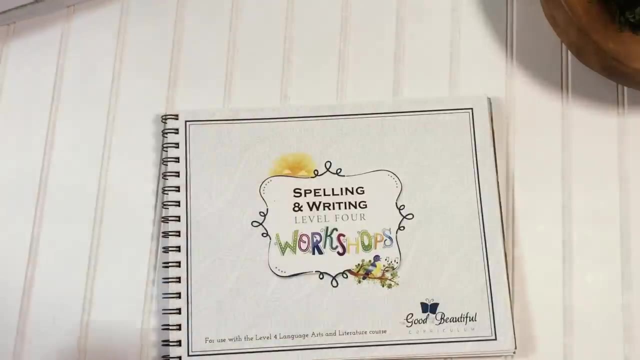 beautiful experience So I want to share with you. first let's look at this spelling and writing workshop. So we did extensive piloting in this course and I'm gonna flip through this as I talk to you about this so you can see this spelling and writing workshops book which correlates with the lessons, So you 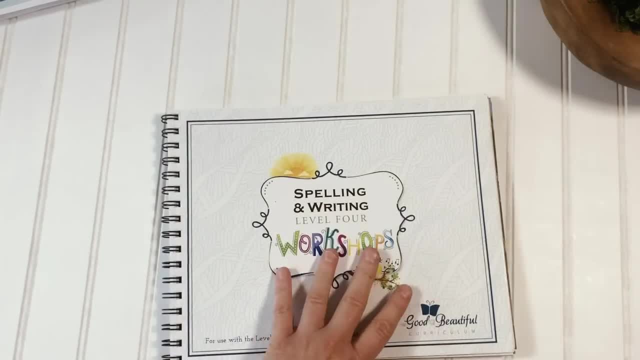 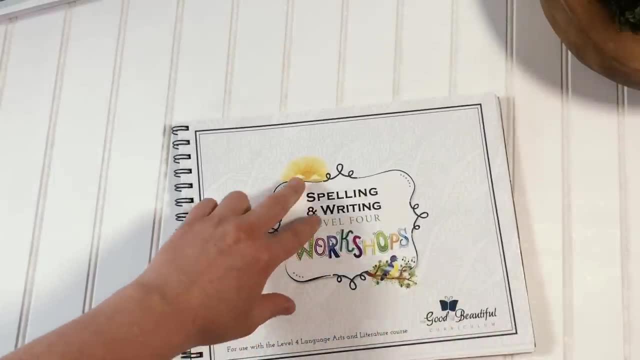 do a lesson in your course book and then it will say: to do a spelling and writing workshop. They do a spelling workshop one day and a writing workshop the next day. So spelling and writing is what we really wanted to make enjoyable and super effective for our children. and we are super excited because our piloting 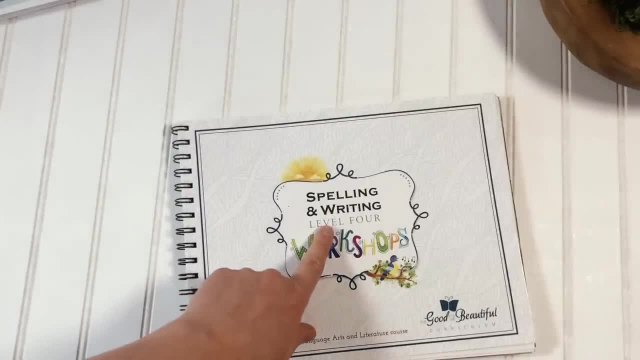 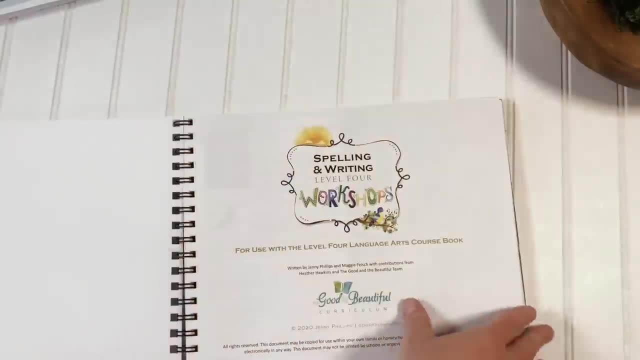 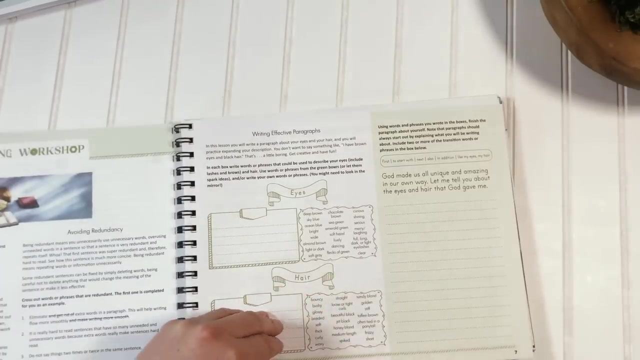 families. that's the number one comment they had is how their writing and spelling improved with their children. They said that their children absolutely blossomed through this course and they would send me samples of what their children are writing. Writing and saying: you have no idea, my child is not, was not a writer. they 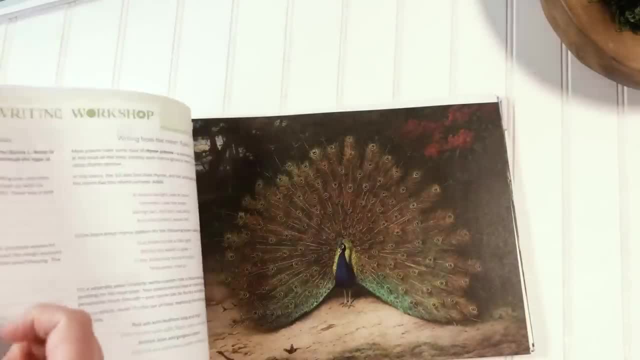 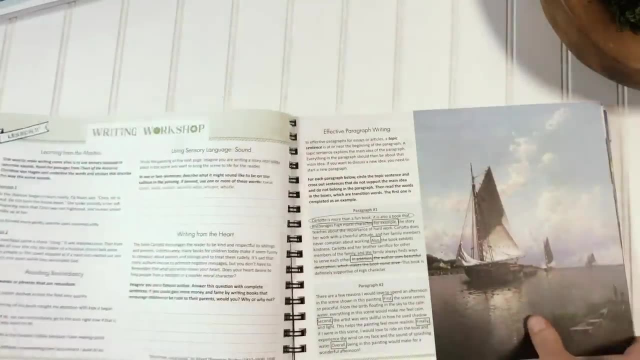 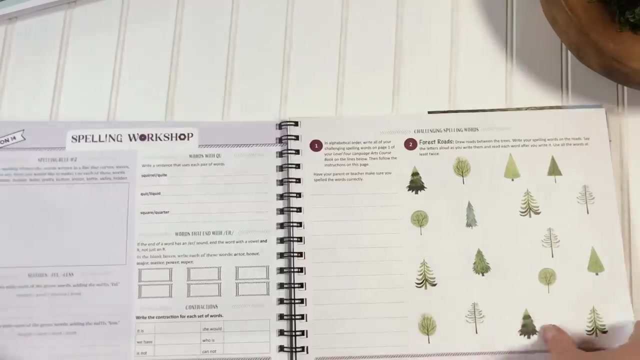 absolutely hated writing, I am. they were just amazed. and one of our pilot families. they said their children did child, did not like writing. and when they were done they asked if they could sign up for a creative writing course because they had loved it so much. And so I am actually having my children in. I teach 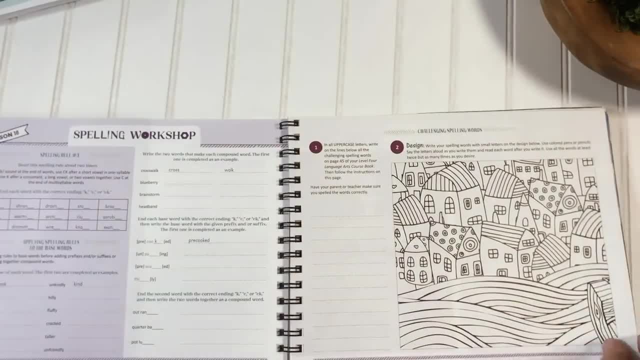 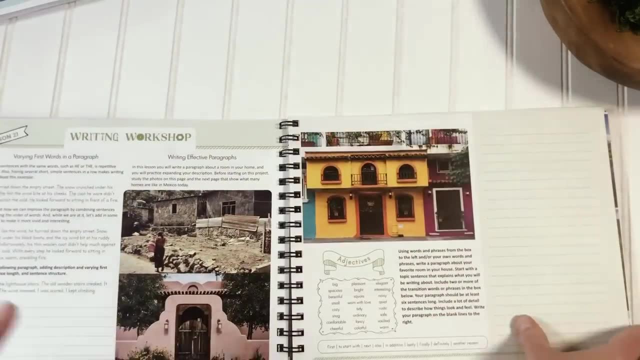 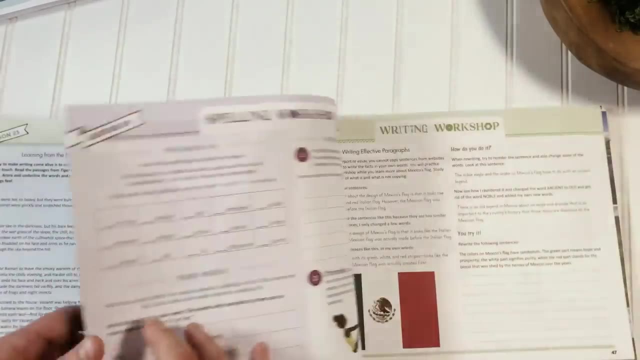 my children home school. my children and a little co-op and I'm having all the children in grades nine and under do this writing workshops book, even though they're beyond level four, just because we feel like the foundation that it creates in writing and in spelling is so important for the children and the joy. 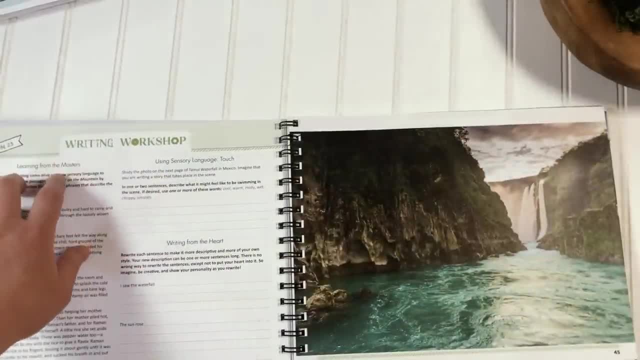 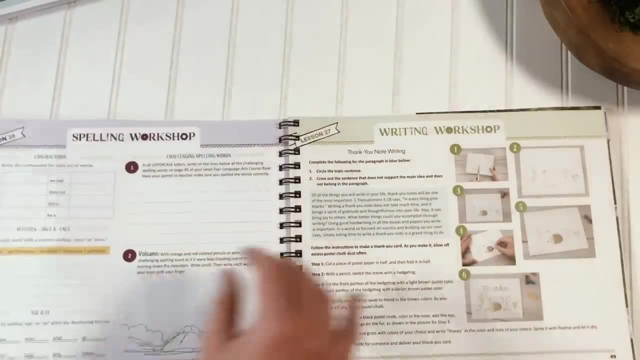 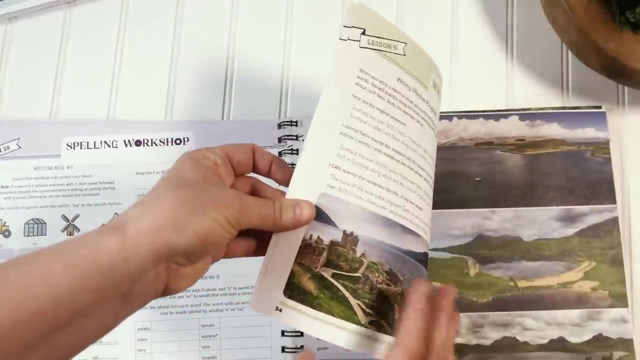 that I have, that it gives them. We have learning from the master sections and writing from the heart sections, which the children absolutely love, as we teach them to write with their own personality and their own creativity and their own, their own experiences. and they are, and they absolutely love it And I won't go. 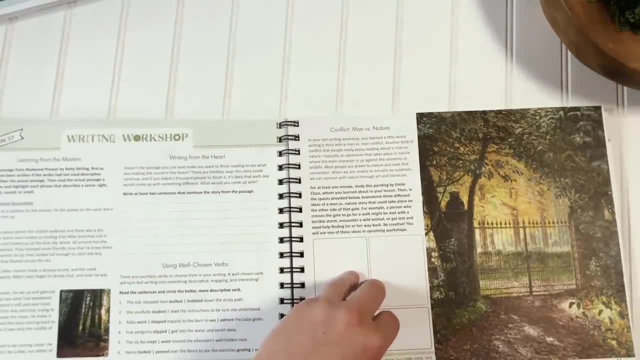 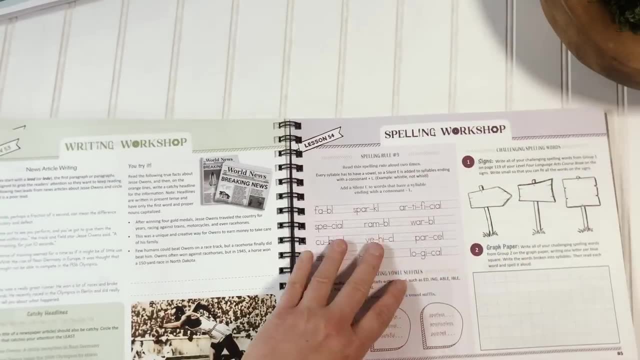 more into how we teach the writing, because I could do a very long video on that, and but I'm really excited about these writing workshops. We have a strong focus on writing, but it is at the level that the child can do. that is not it does. 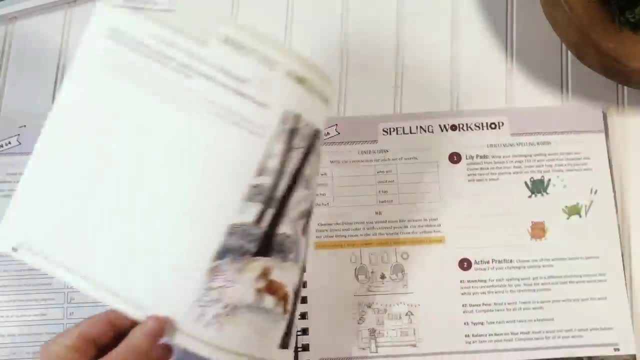 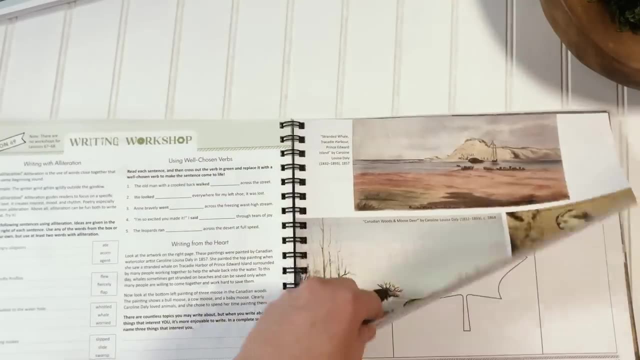 not overwhelm them. That's one of the things that we look for, the pilot family. if a lesson overwhelmed the children, we would rewrite it until the children loved it, till all the pilot families came back and said: yes, my child loved doing this, he totally got it, and it was a quite a laborious. 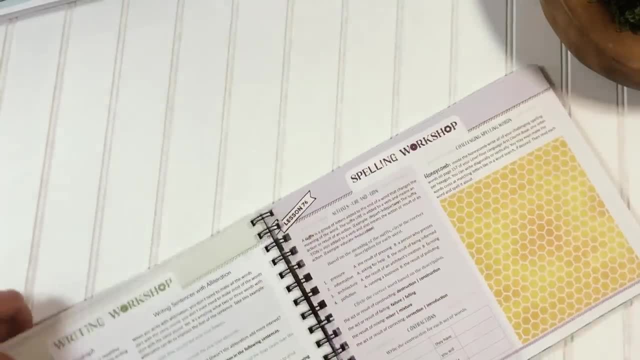 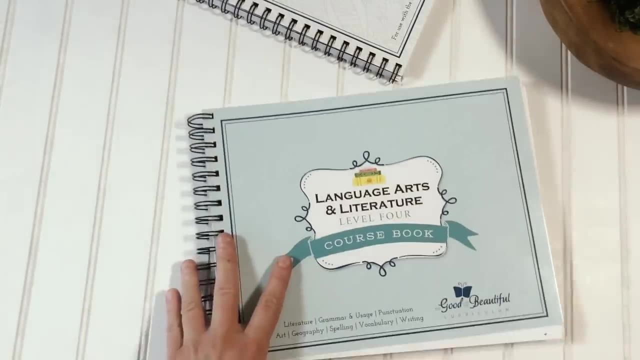 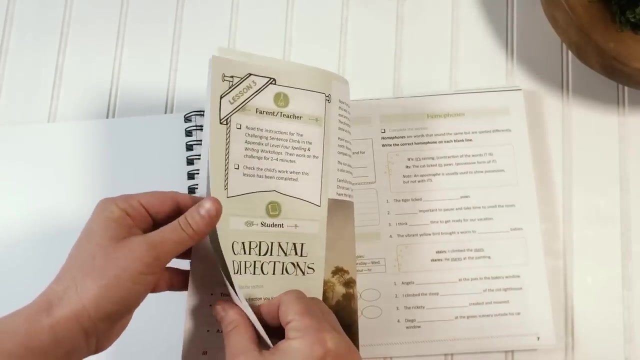 process, but we're really excited with the result. Let me give you a quick flip through of the course book here and tell you how the lessons work. So the lessons take about five to seven minutes. So the lessons take about five to seven minutes for the parent to do with the. 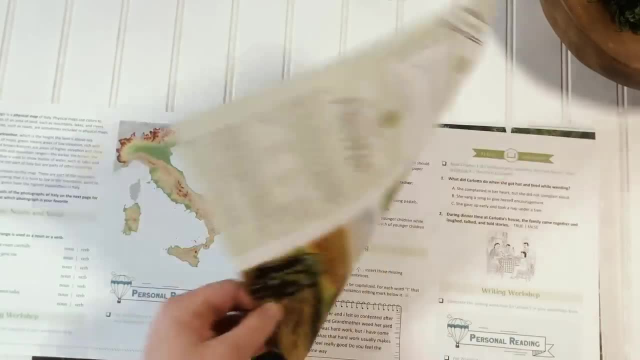 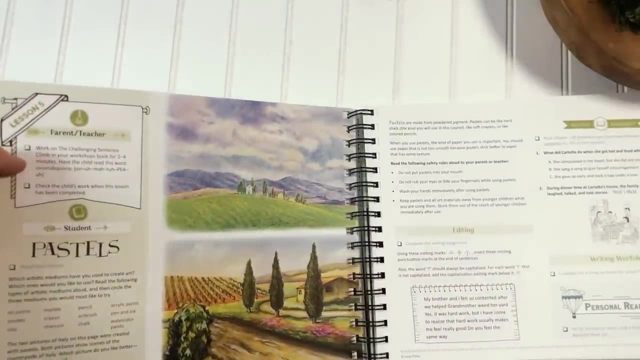 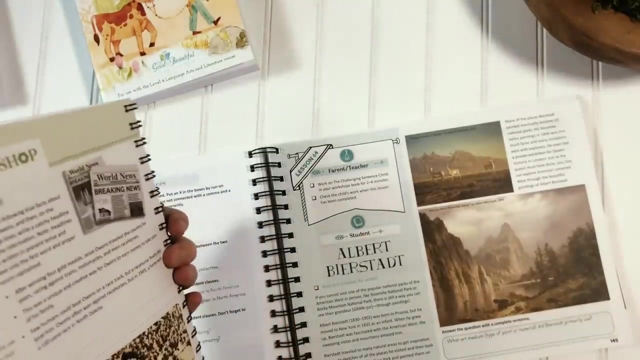 child and they will do this little parent teacher section here, which is either to work on the challenging sentence climb which is in the back of your workshops book here. These used to be flash cards- challenging word flash cards- but we found with our pilot families that this was a very effective 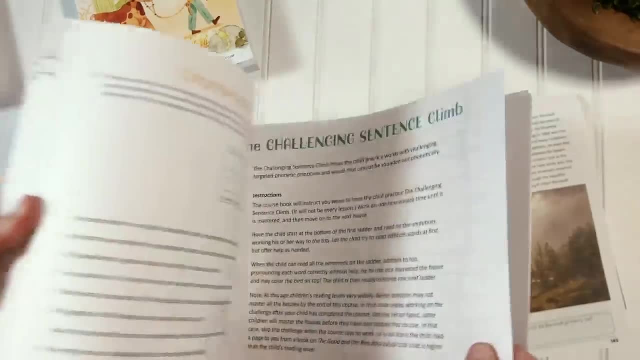 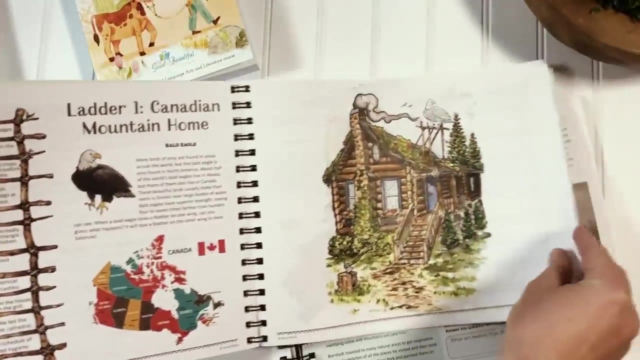 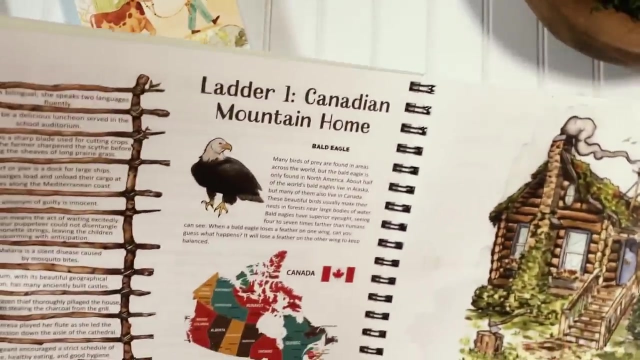 way to do it. So they have this challenging sentence climb. that gives you a short time here, but basically they have these different ladders from different homes. so this is a Canadian home and when they master this ladder then they get to color in this bird there which they read a little bit about. so we have these. 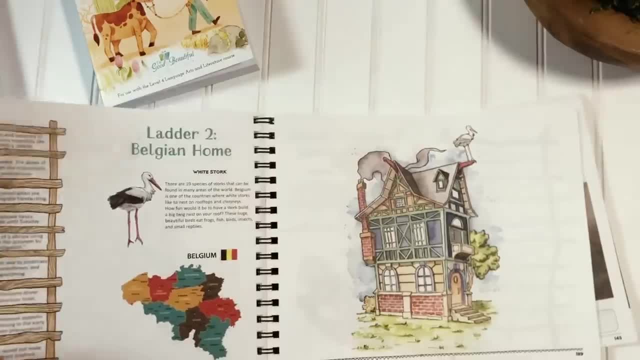 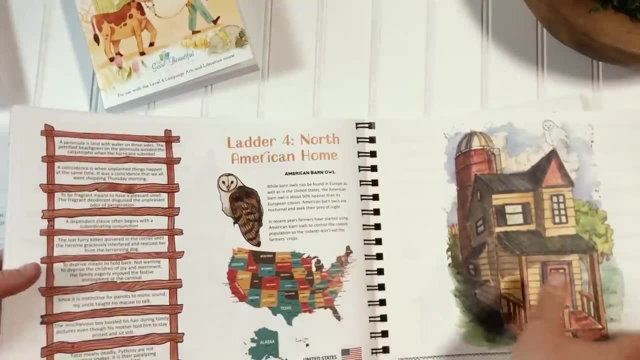 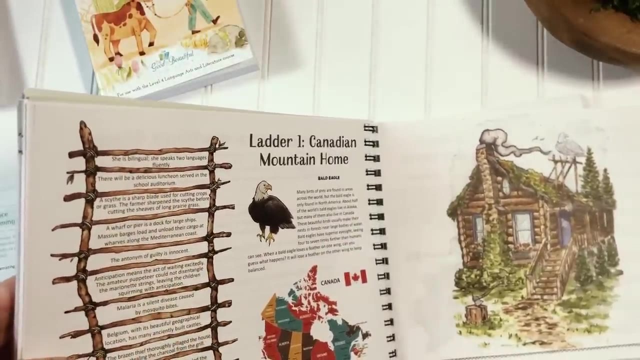 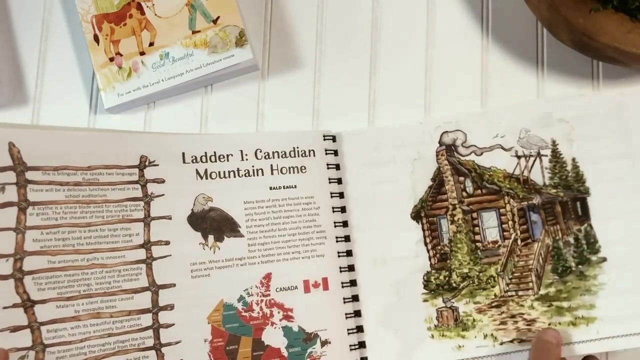 different homes from different countries, so this one is Belgium and we have South Africa and North America and different ones. so the kids think it's really fun, and in here are so many difficult words to pronounce that can't be sounded out very easily and this is really going to help the children be exposed to a ton of 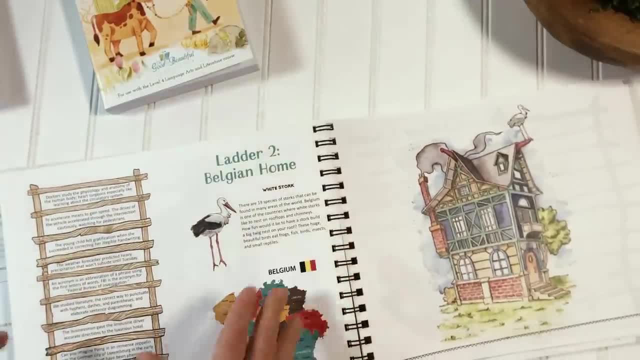 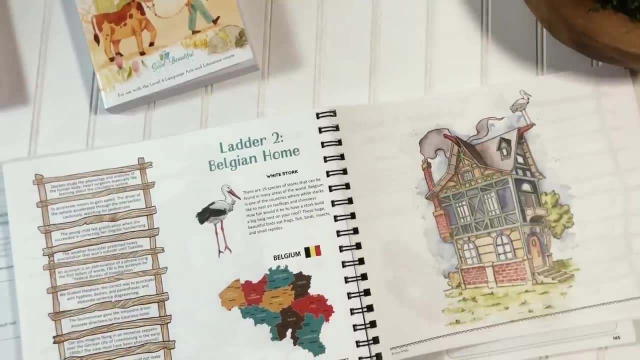 words that they can practice. when children get into level four, they still need help in increasing their reading skills. so we don't do direct phonic instruction anymore. that ends in level three. but they still need to improve their reading skills and if they're just reading books on their own, 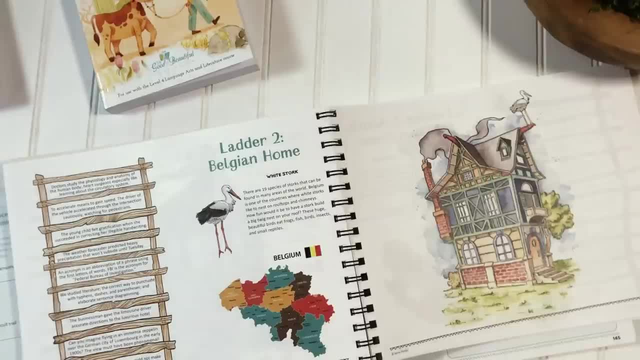 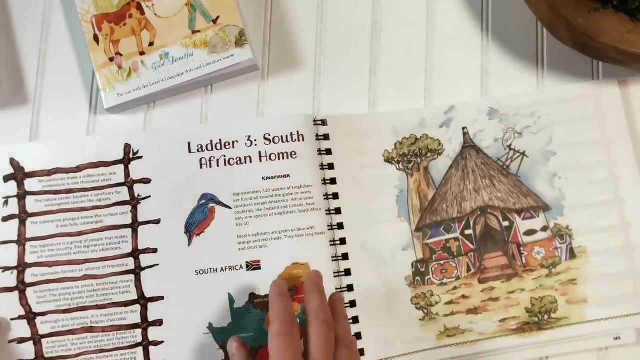 to themselves. it's going to be hard for them to improve because they're gonna skip over those hard words, and so we have concentrated all of these hard words in this fun way. so you're just gonna try to climb the ladder and see how far they can get in two to four minutes, and then you'll master the. 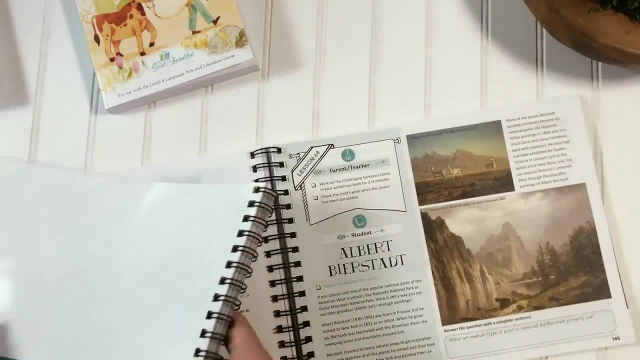 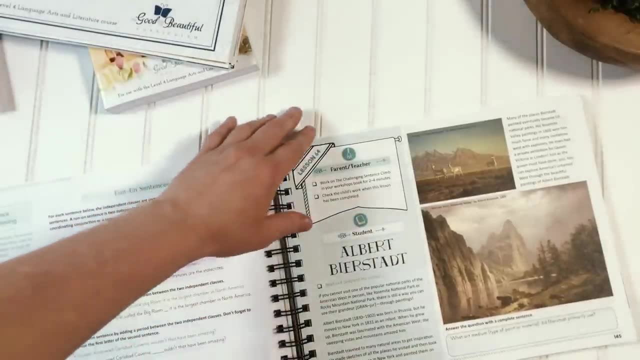 different ladders, and so that's about in every other lesson that you will open up and do that. so it says work on the challenging work time and then check the child's work and that's all the parent has to do and then they're gonna read. 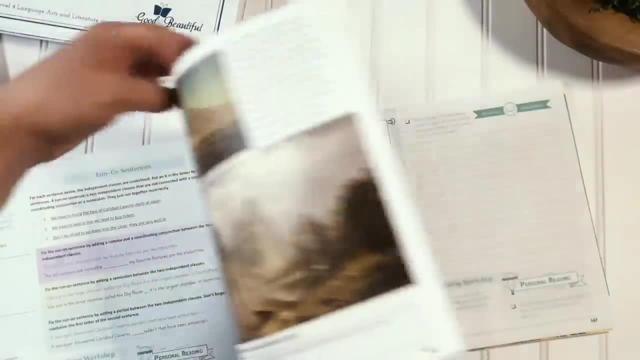 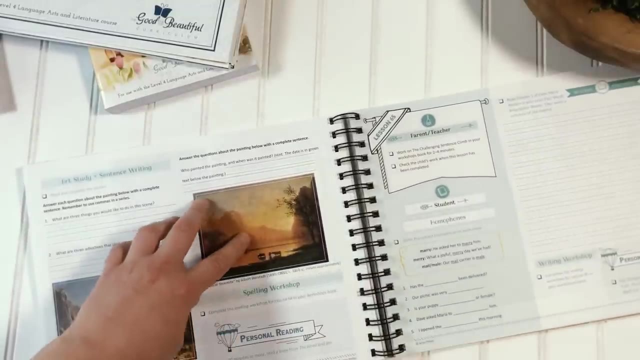 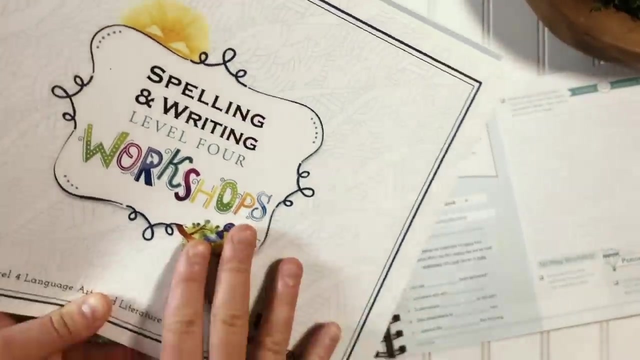 about this artist who painted and national parks, because that is what we're talking about. and then, as they're doing their exercises, they're studying some more of the art. and then it says to do their spelling workshop. so they're going to open up their spelling workshop and work in here. we also suggest that they do personal. 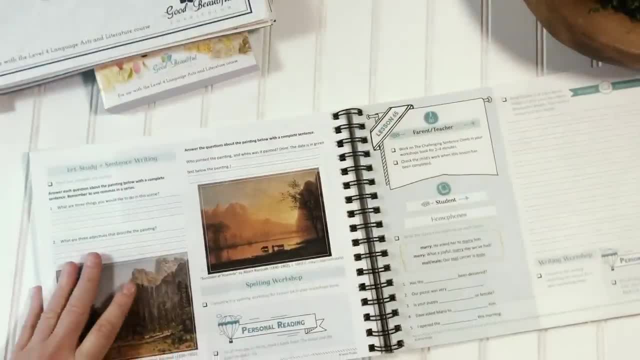 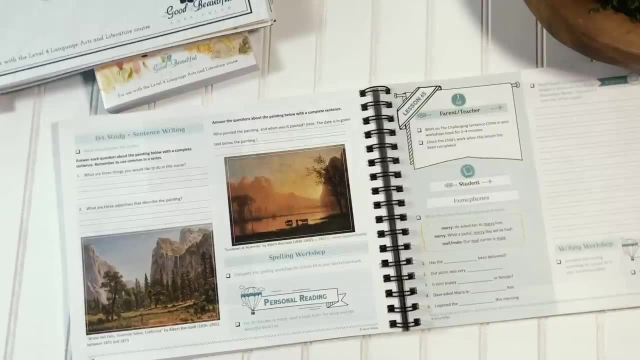 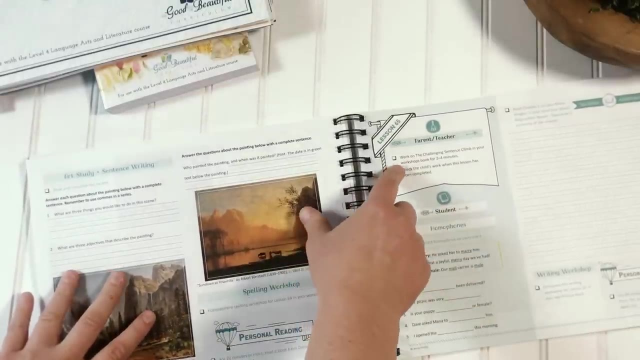 reading for at least 20 minutes a day from books from the good and beautiful book list, but that can be done anytime, even at night or, um, you know, before they go to bed, or or anytime that you want. so the lessons take an average of 30 minutes and the parent portion is between two, two and seven. 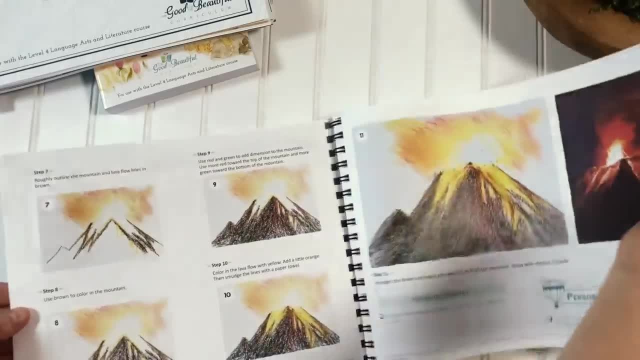 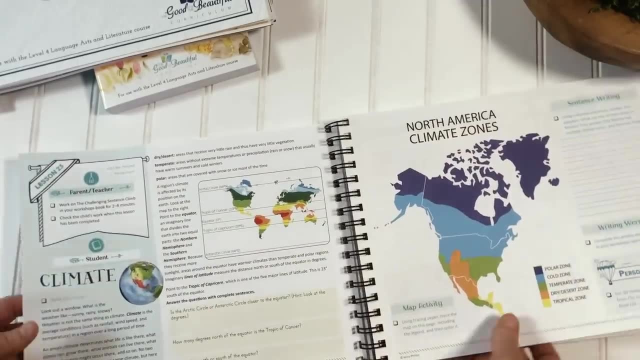 minutes. there's also some sections. here's the volcano. this was a hit with our pilot families. there are also some sections. i'll just do a little clip through, uh, flip through here, um, while i am looking for some sections where the child is going to read larger sections. 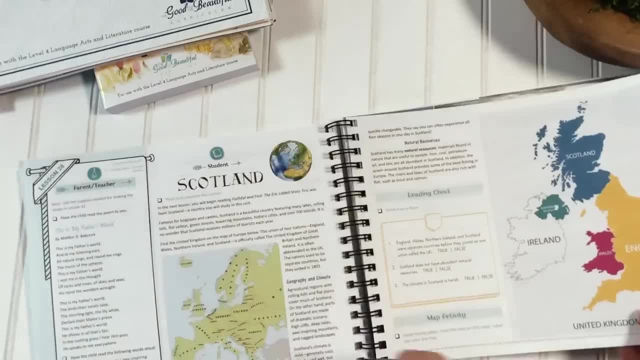 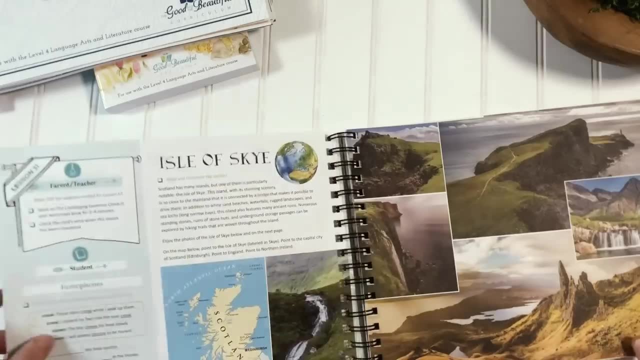 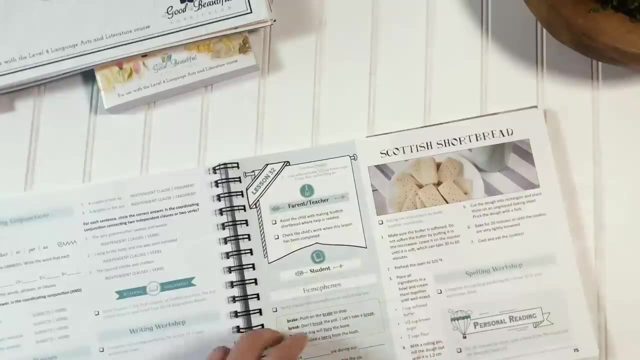 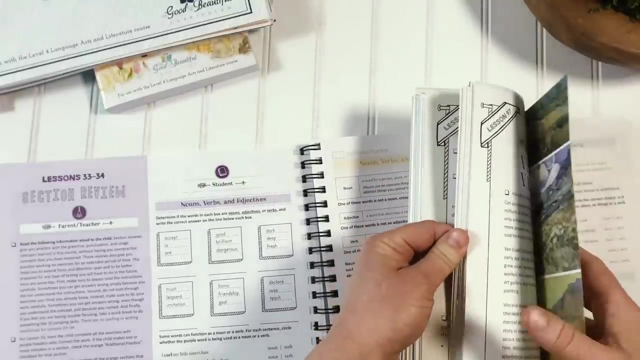 um to the parents. so scotland- this is when they are reading the story of eric little in their biography and he was from scotland and, uh, they have a few recipes that they do. so there is some scottish shortbread that they do when they're studying scotland and they do a yogurt cake- this one, the families and kids. 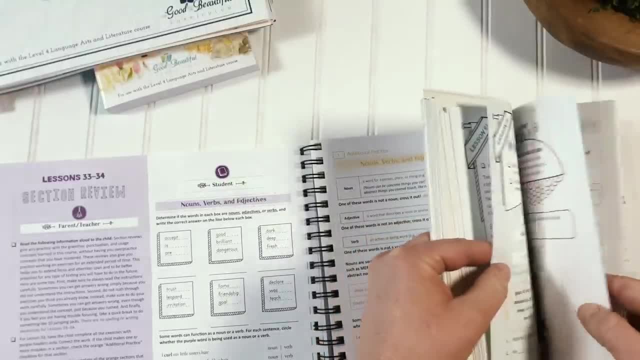 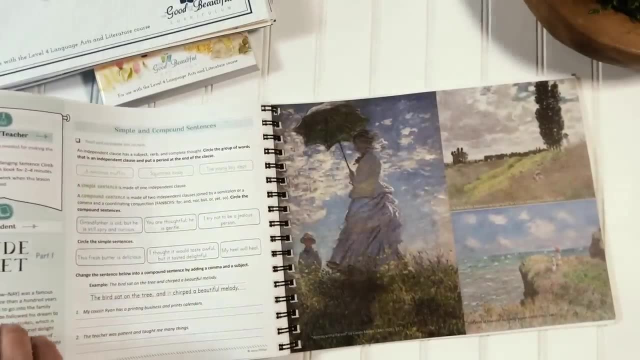 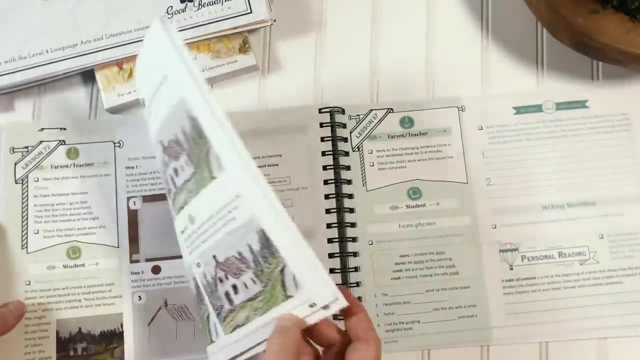 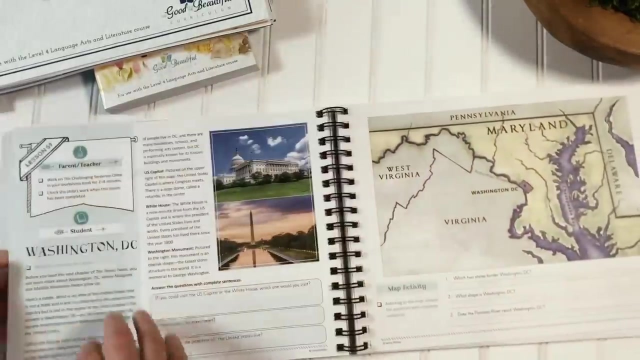 absolutely loved and it's super easy. um, they absolutely loved it, so they do this um yogurt cake. but i'm going to flip through this way and show you they do study, study um club monet and the area where he lived. so let me see if i can find some of these sections here where you're. 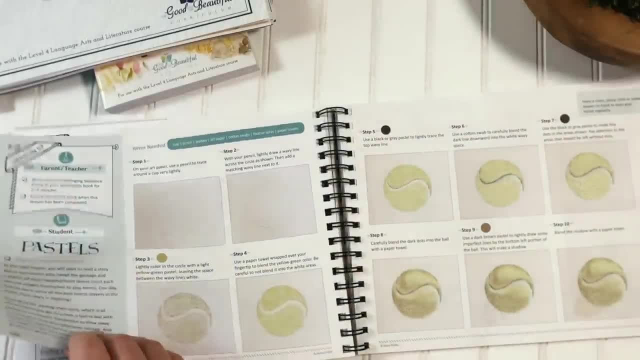 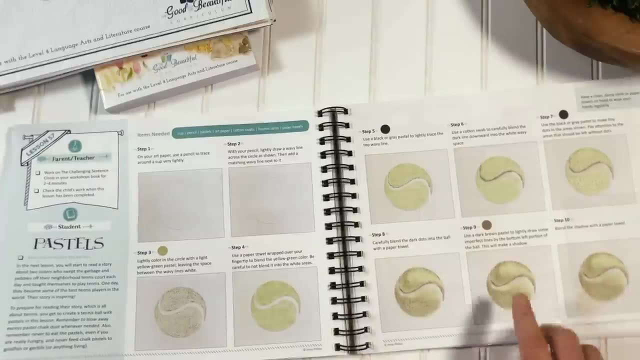 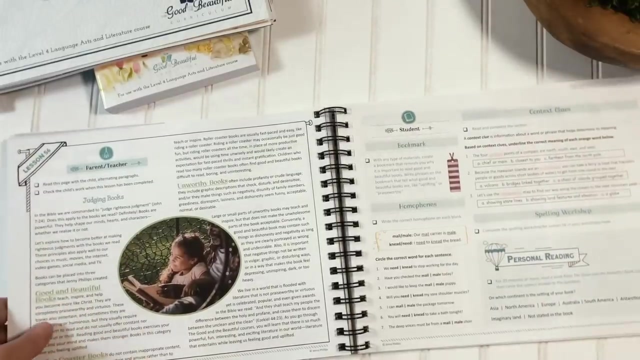 going to read to the parent. this is where they're reading about these two african-american sisters whose story has never been published before. we were super excited to publish it, um. who were amazing tennis players, um. so here's an example of there are some sections where the parent will read.